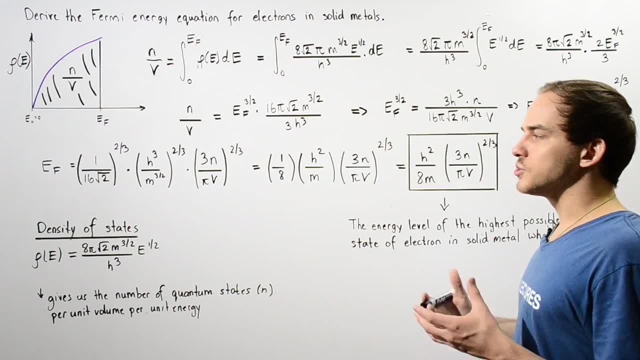 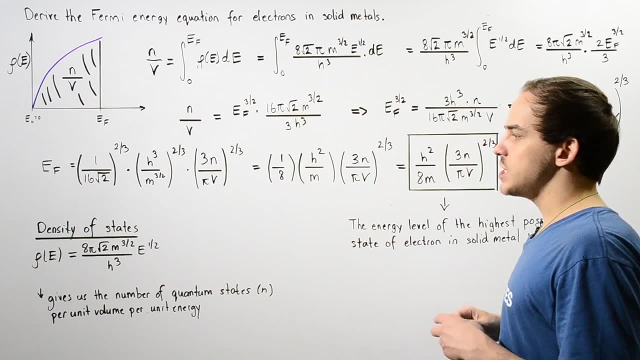 and we bring that solid metal to a temperature of zero Kelvins. So now we want to derive the equation that will give us the Fermi energy of our electron within that situation. Now, to actually derive the Fermi energy equation for electrons in solid metals, we're going to 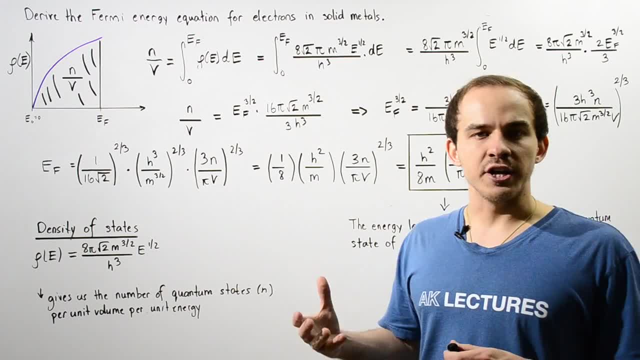 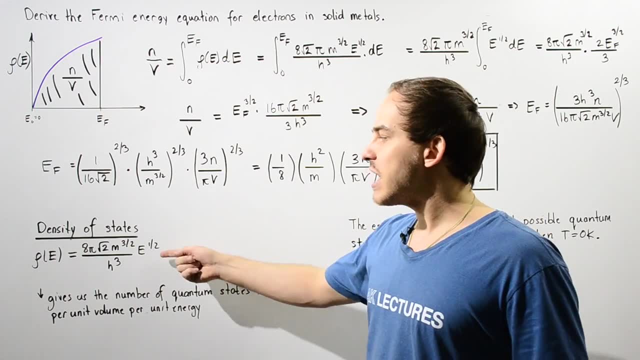 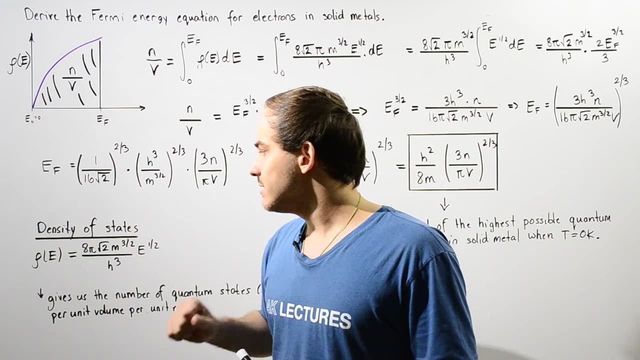 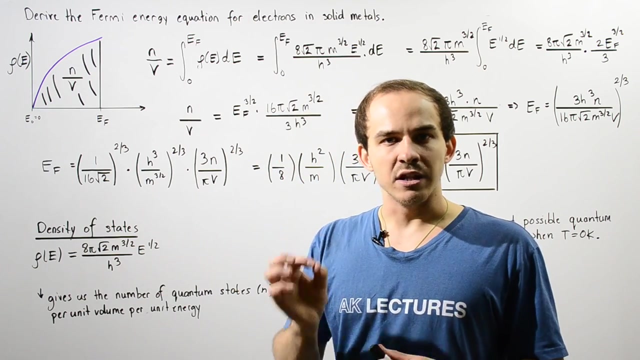 use an earlier result. We're going to use the density of states function. So basically, this is a mathematical function that is given by the following equation: So rho, which depends on E, is equal to this entire quantity. Now this basically gives us the number of possible. 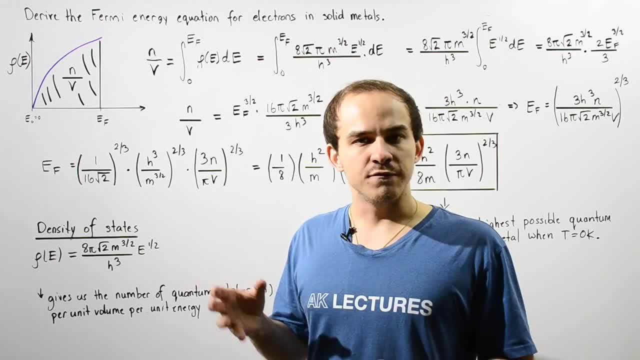 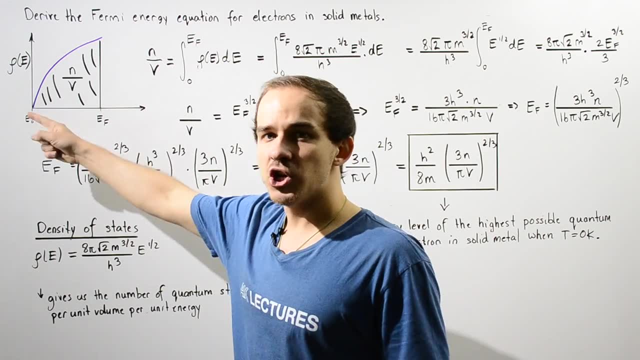 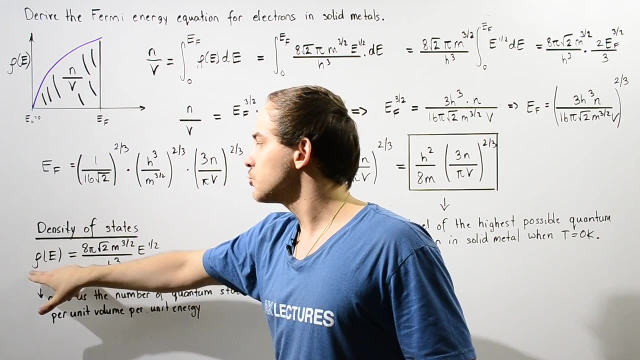 energy, quantum states of the electron per unit volume, per unit energy. And we're going to derive that energy Now if we plot this equation on the xy plane as shown, where the x-axis is the energy of the electron and the y-axis is our density of states, function, rho of E. 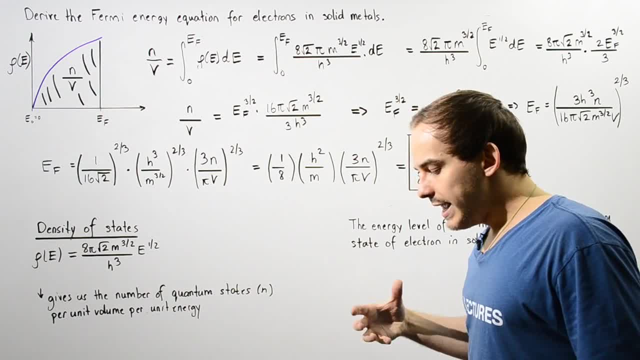 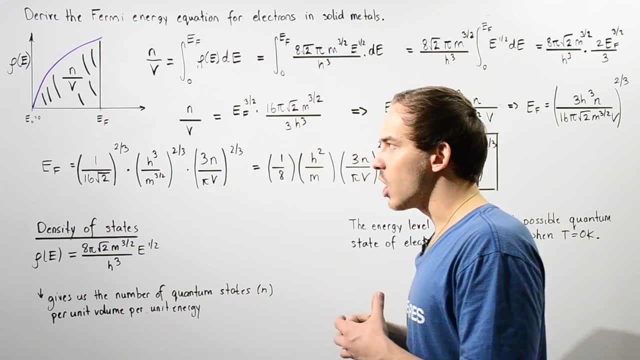 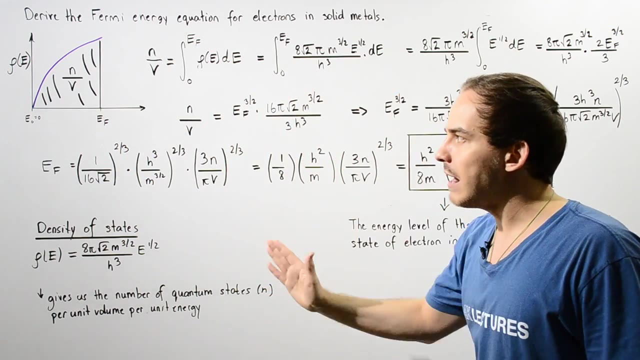 we get the following purple curve. Now, if our energy, if our temperature of our solid metal is brought to absolute zero, that means the highest possible quantum energy state that our electron will be found in is given by EF, which corresponds to the Fermi energy level. So 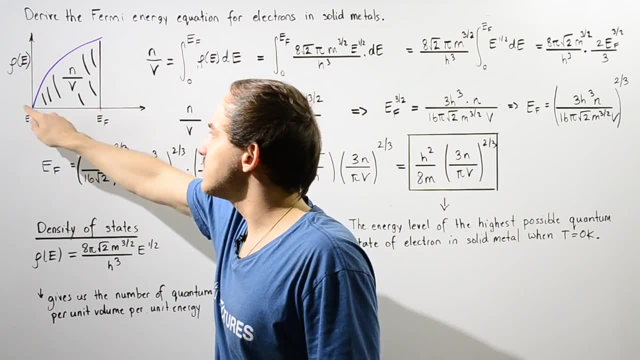 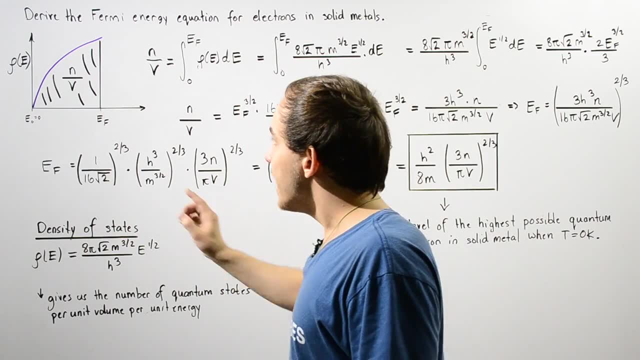 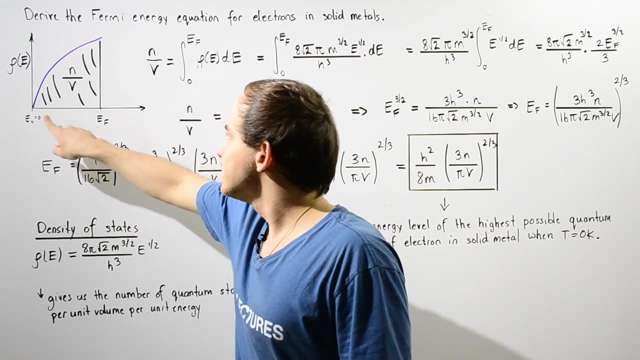 basically, this is the highest possible value and this is our lowest possible value. We're going to choose this to be equal to zero. Now, if we integrate, if we use calculus and integrate this curve from this lower bound to this upper bound, we get the shaded region which corresponds. 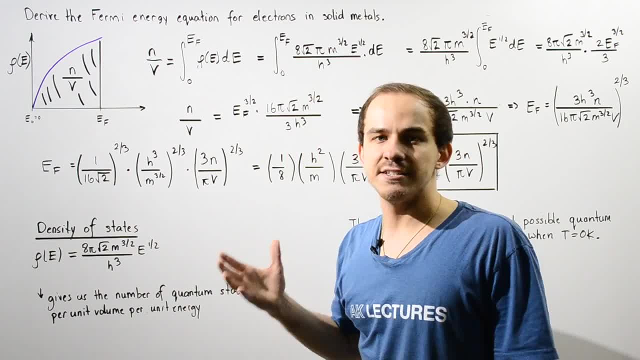 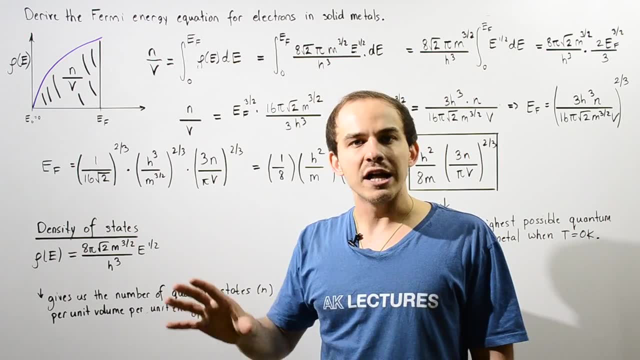 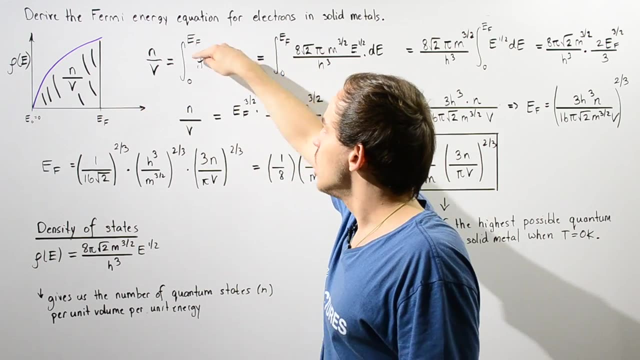 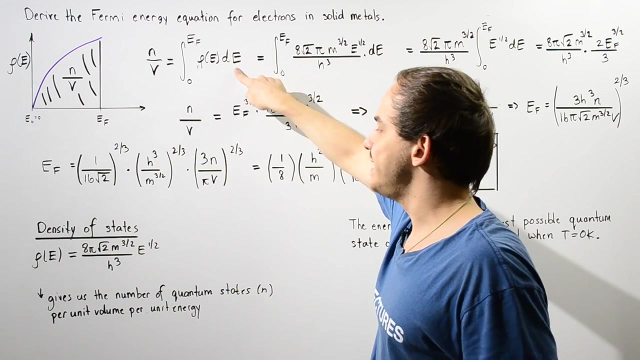 to lowercase n divided by uppercase V. So if we integrate this function we get the number of possible quantum states per unit volume. So we get n divided by V is equal to. we take the integral from our lower to the upper bound of this function with respect to dE And notice the per unit energy. 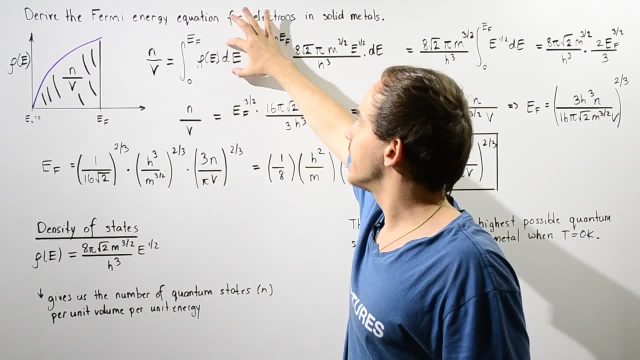 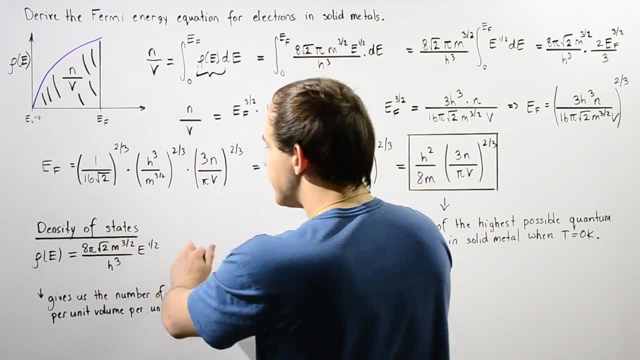 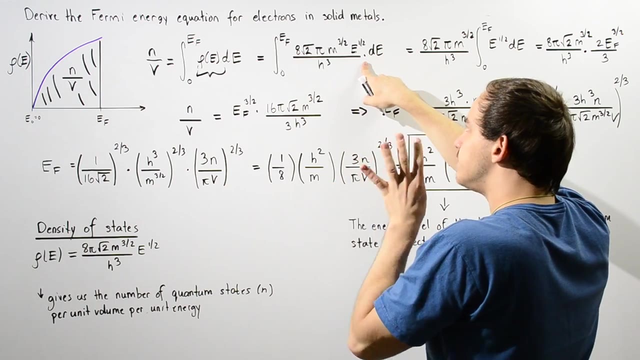 term cancels out, because we're essentially multiplying by our energy term. So let's actually take this function and replace it with this entire equation to get the following result: And now we can take our constant values and bring it outside of our integral. So we bring outside. 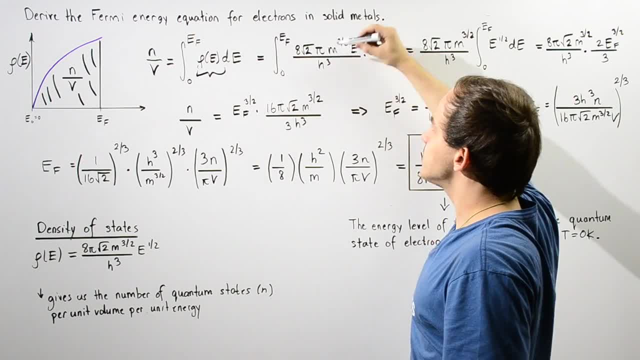 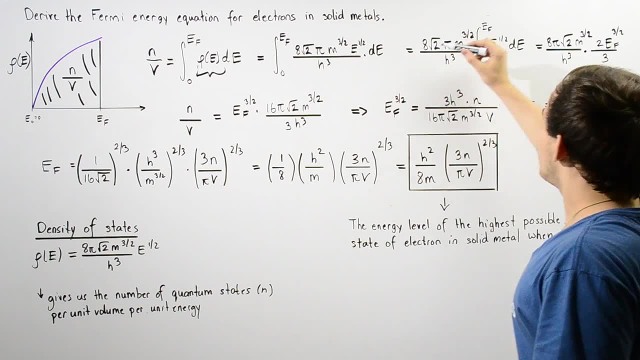 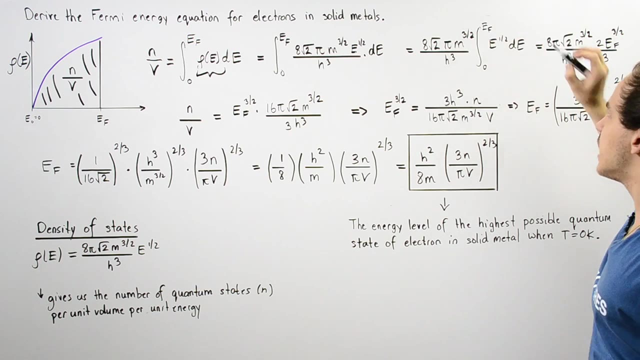 the 8, the radical, to the pi, Planck's constant, as well as m, the mass of our electron, And we are left with the following result: So we're basically multiplying the constant by the integral, from zero to our Fermi energy level, and we're integrating this. Now, if we actually integrate, 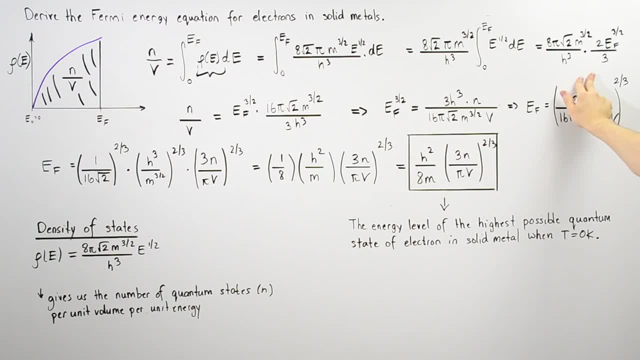 and evaluate that integral, our result is as follows. So we see that n divided by V is equal to this quantity, which can be rewritten in the following format: So now, because we're looking for the equation, we're going to be able to get the number of possible quantum states per unit. 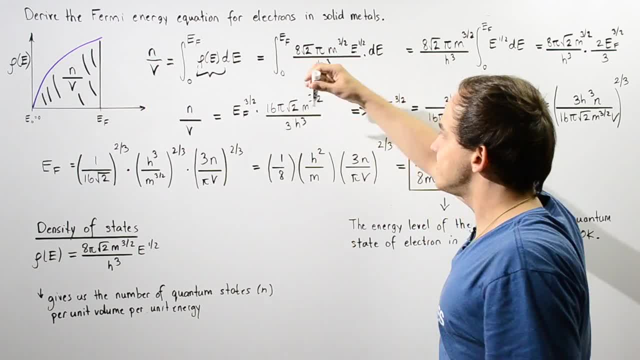 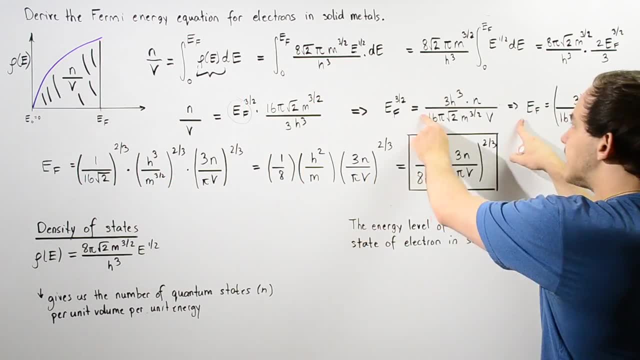 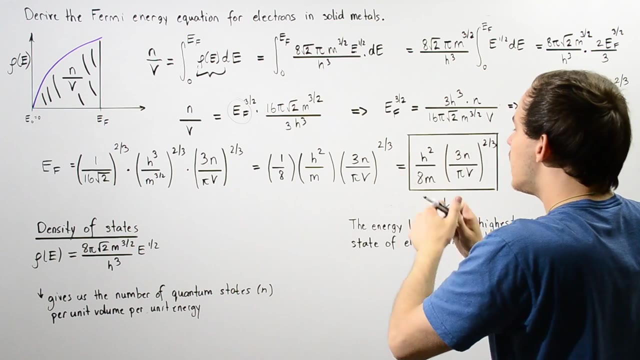 equation for the Fermi energy. We basically solve for this quantity. So we bring this entire term to this side and we get the following result: And now we basically raise both sides to the power of two, and then we raise both sides to the power of one third And we get the following result: 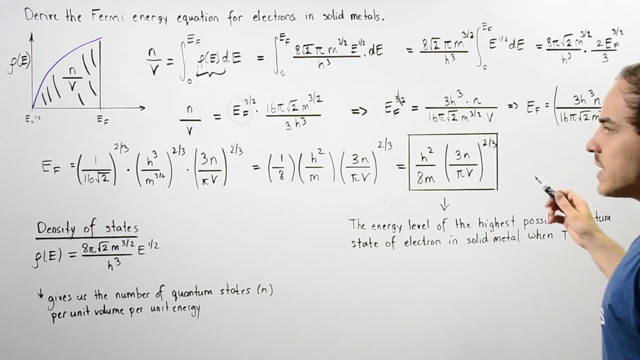 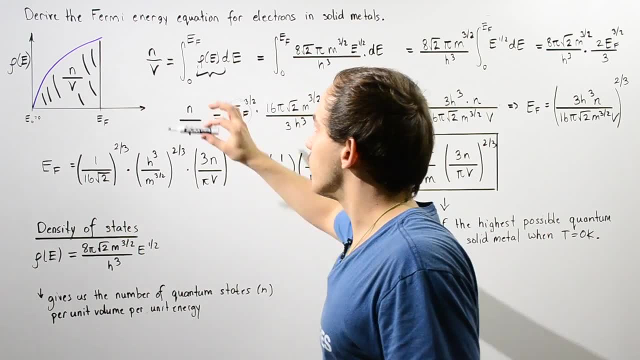 and this cancels out. So let's take this and let's rewrite it in a slightly different way. So let's take this and let's rewrite it in a slightly different way, As shown in the following section. So our Fermi energy EF is equal to. so we raise this to the 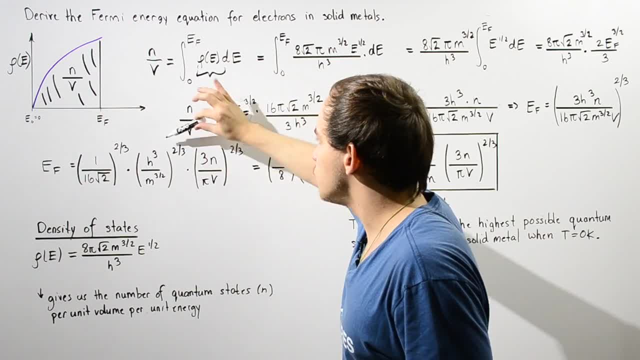 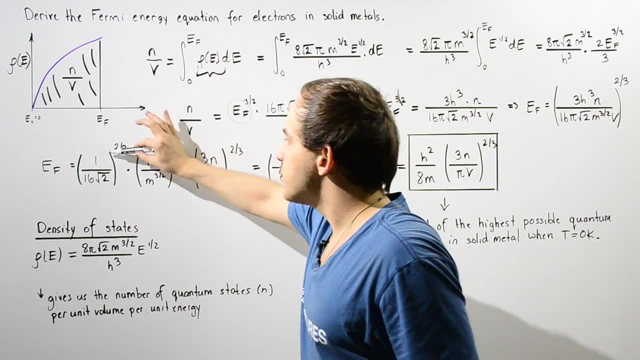 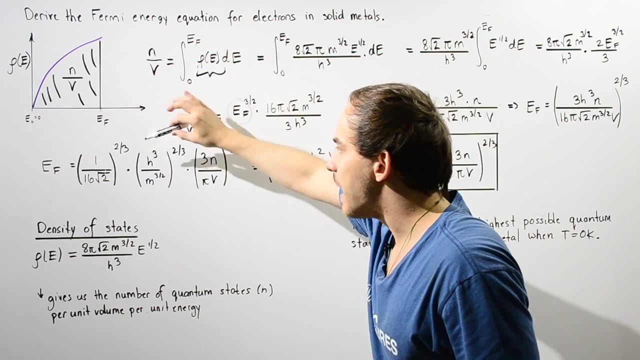 power of two thirds. we raise this to the power of two thirds and this to the power of two thirds. So, basically, we take this and split it. So notice: this simply gives us one divided by eight. this simply gives us H to the power of two divided by M, and this: 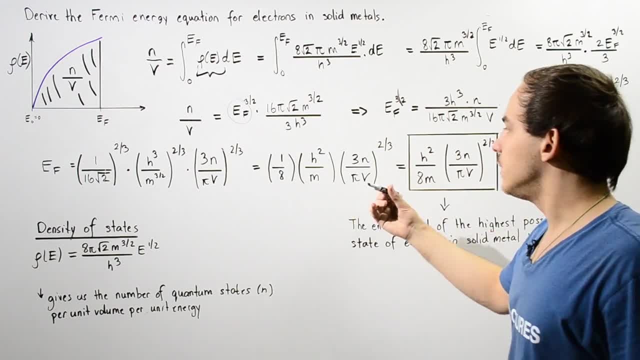 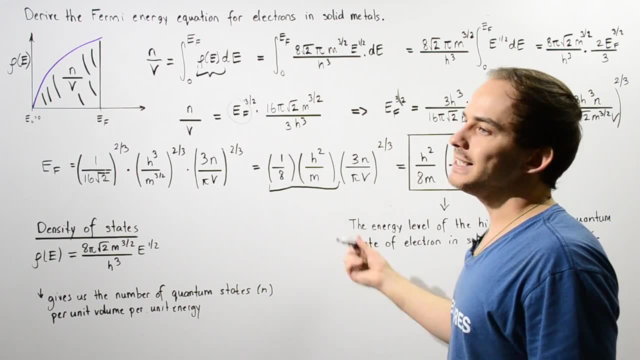 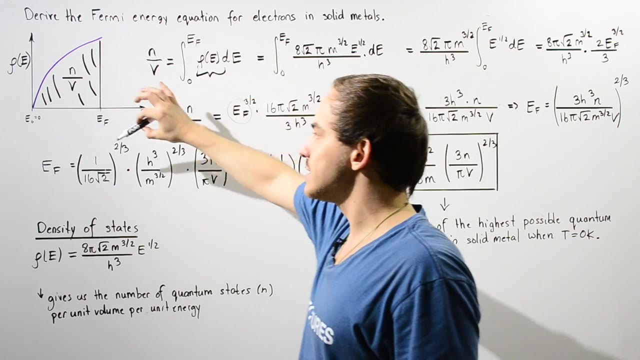 we leave it as it is And we get the following result. So now we can combine these two terms and we get the following equation that we defined in the previous lecture. So this gives us the Fermi energy given by this quantity of our electron in the highest possible energy quantum.